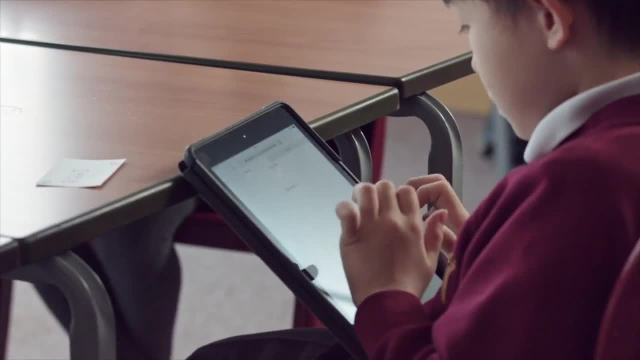 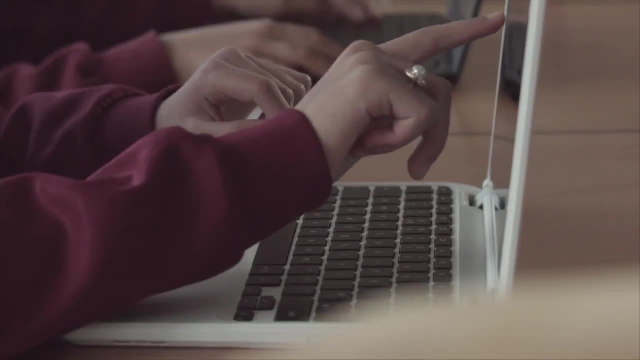 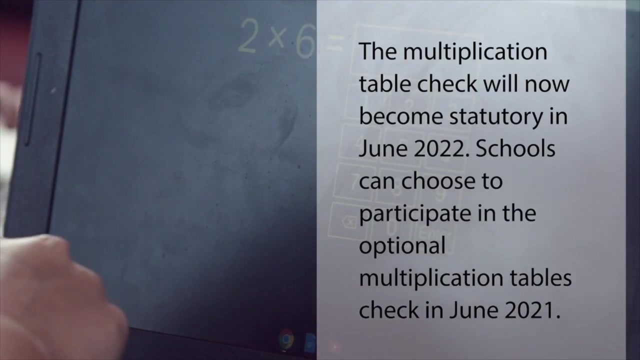 in England, Announced by the Department for Education in 2016. the check is intended to support teachers in ensuring that all children know their times tables by the end of primary school. Schools across the country will be required to administer the check for the first time in June. 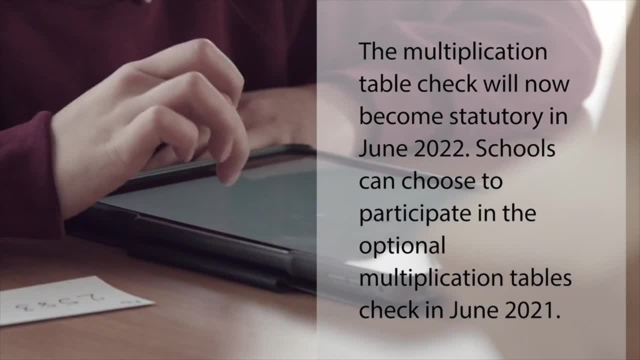 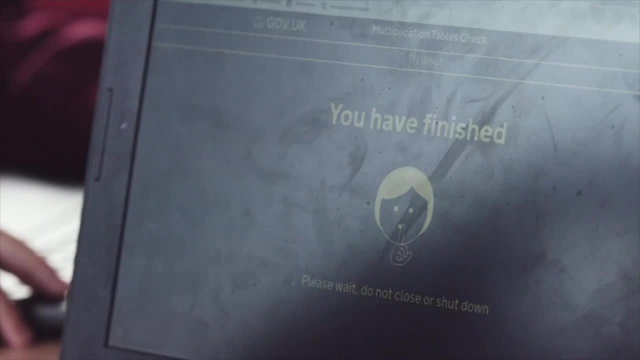 2020.. The check will assess whether Year 4 pupils can recall their times tables to 12 fluently in a series of 25 questions and will take most children no longer than five minutes to complete. The Check will also assess whether children are able to recall their times tables. 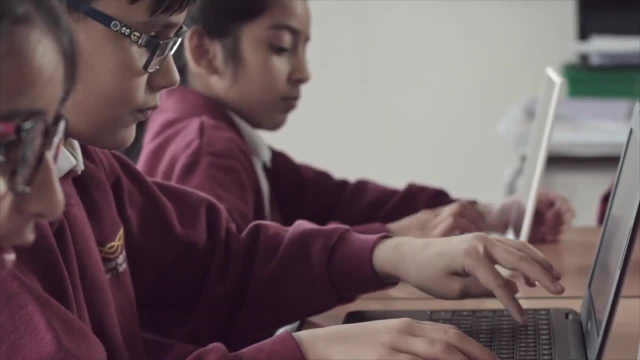 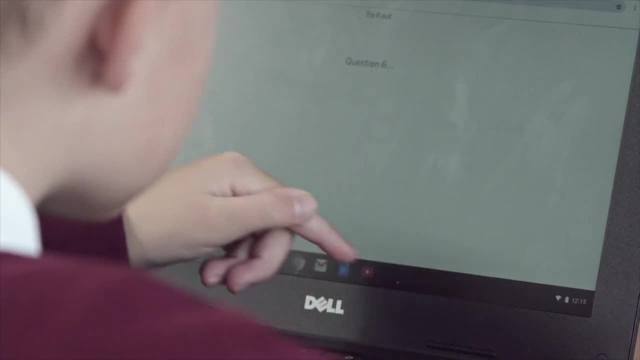 to 12 fluently in a series of 25 questions and will take most children no longer than five minutes to complete. complete It has been developed working with over 2,500 primary schools throughout England. This has included extensive user research and trialling involving over 14,000 pupils. 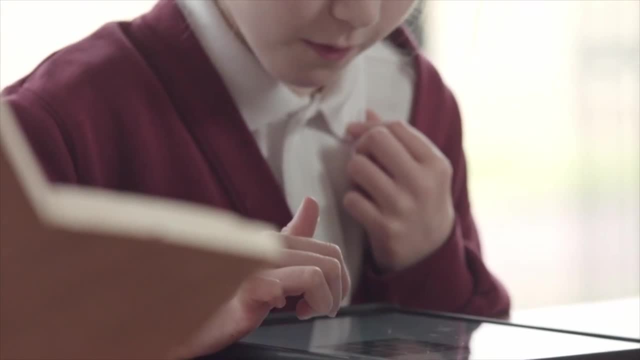 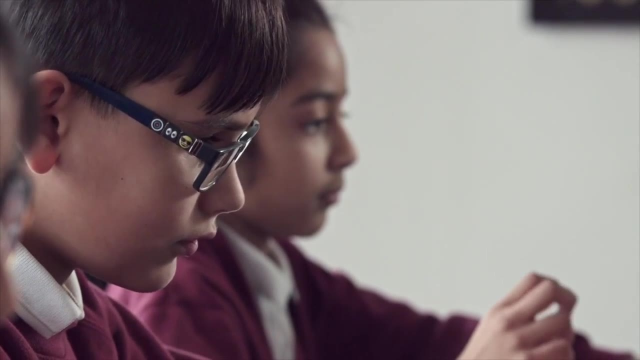 over the last three years. Once the check becomes statutory, schools will be required to report the results to parents or carers. From the results, schools will be able to identify those pupils who may need more support with their times tables. They will also be 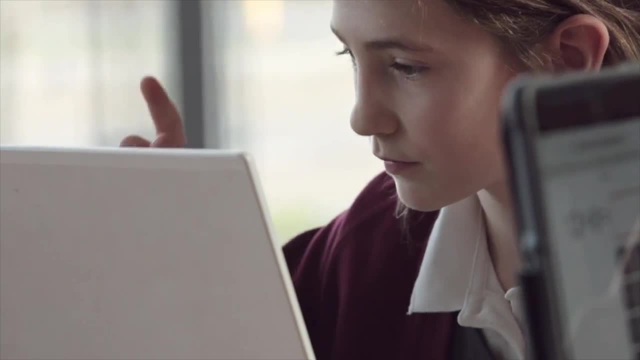 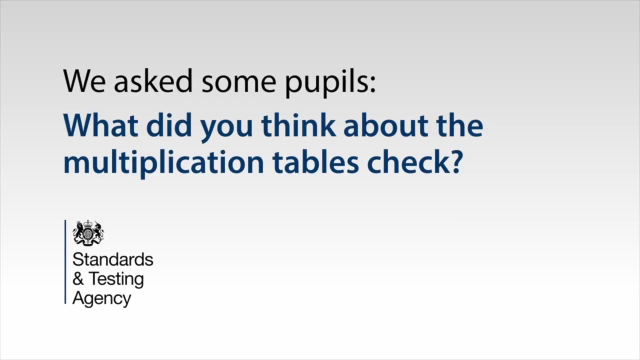 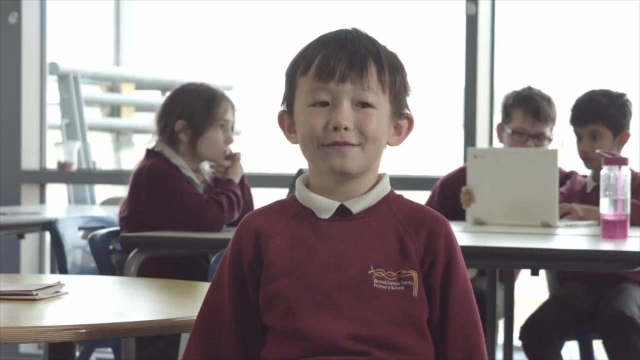 able to determine how their pupils' performance compares to national and local authority-wide averages and identify any areas for improvement. The team that put this together did a very good job. It's more exciting because it's on a computer. I thought it was quite fun because it was a bit different to all of the other checks. 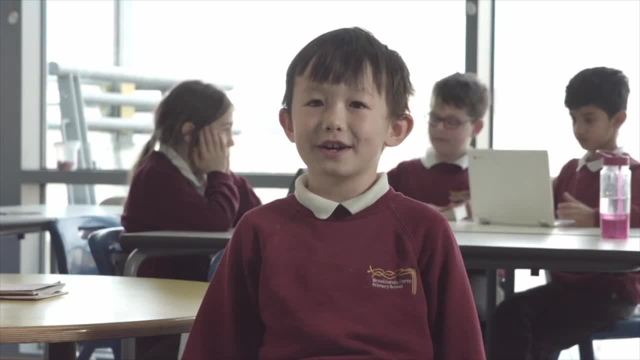 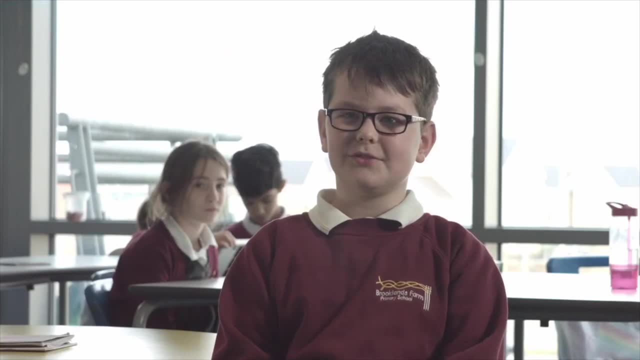 or quizzes that we do because you actually get to go on the device. It was fun because we don't usually get to go on devices and we got to go on devices to start. I think the kids in school will like it. I'm going to tell all my friends. 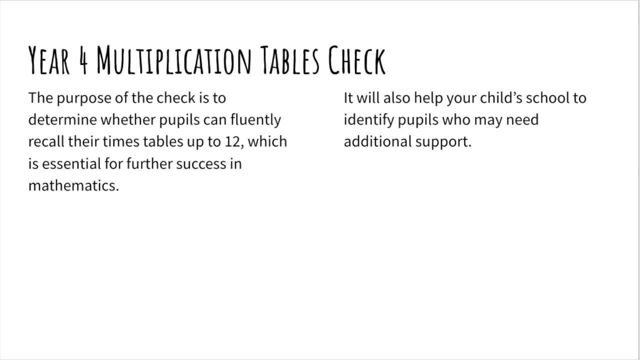 The purpose of the check is to determine whether pupils can fluently recall their times tables up to 12, which is essential for further success in mathematics. It will also help your child's school to identify pupils who may need additional support. Ofsted have stated that pupils without 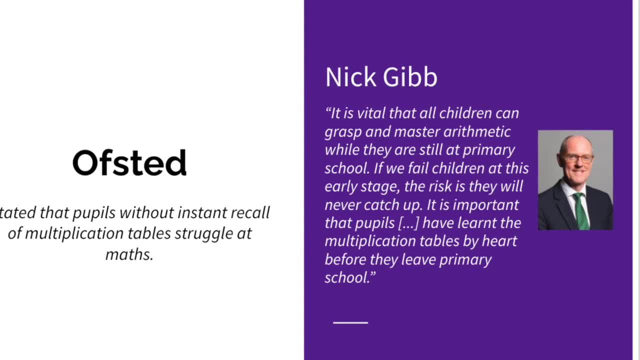 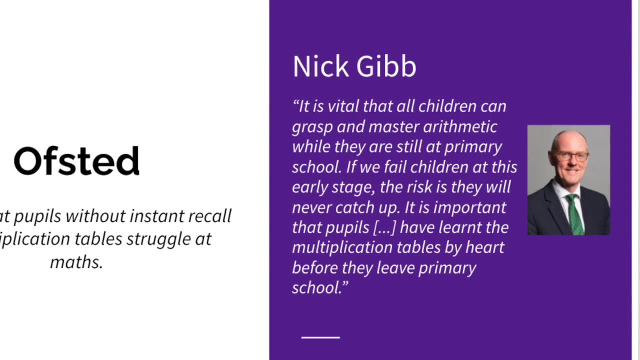 instant recall of multiplication tables struggle at maths. Nick Gibb, the school's minister, has also said that pupils who have no record of multiplication tables struggle at maths. He also said that it is vital that all children can grasp and master arithmetic while they 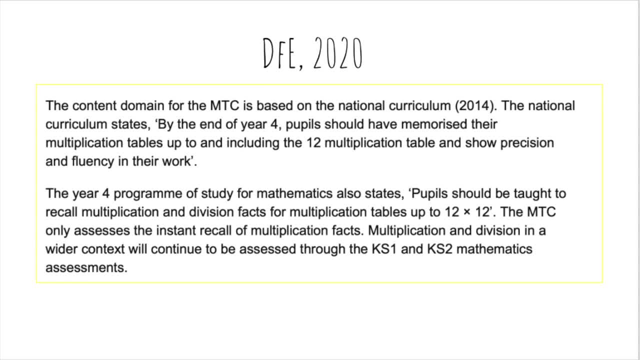 are still at primary school. The Department for Education states that by the end of year, four pupils should have memorised their multiplication tables up to and including the 12 multiplication table and show precision and fluency in their work. So it is absolutely vital that we provide the support that pupils need to make sure 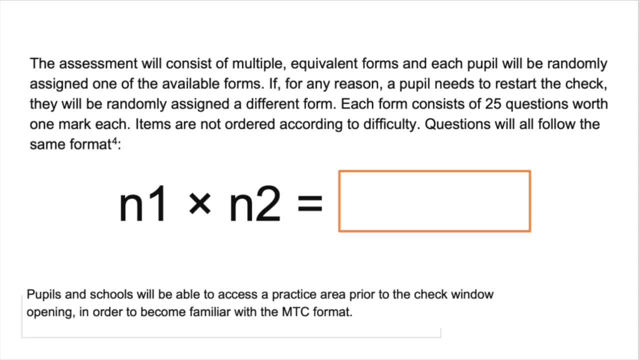 that they are able to do this. The assessment consists of 25 questions worth one mark each. Items are not ordered according to difficulty. Questions will all follow the same format. The example shown on the screen represents number 1 multiplied by number 2.. Pupils will then be able to access a practice. 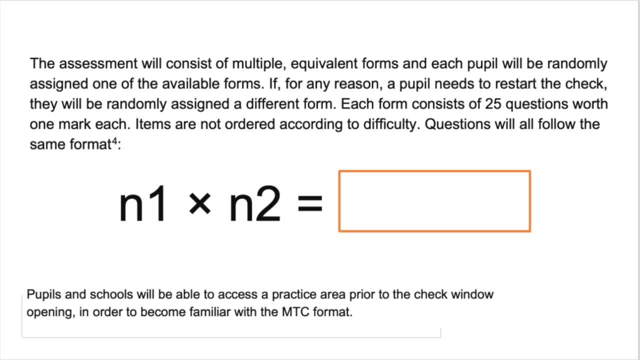 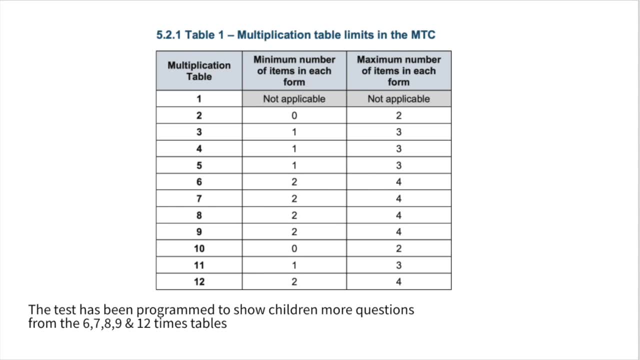 area prior to the check window opening in order to become familiar with the MTC format. This table shows the multiplication table limits in the multiplication tables check. As you can see here, the test is geared towards the 6s, 7s, 8s, 9s and 12 times tables. The 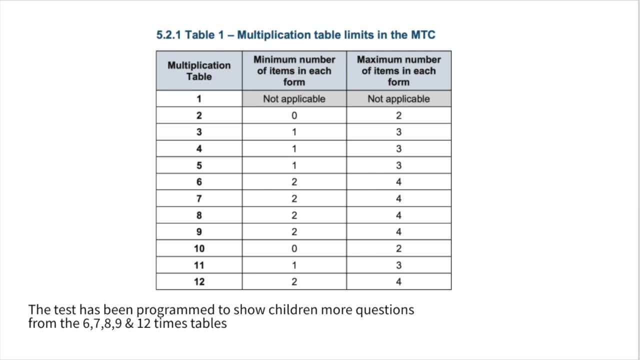 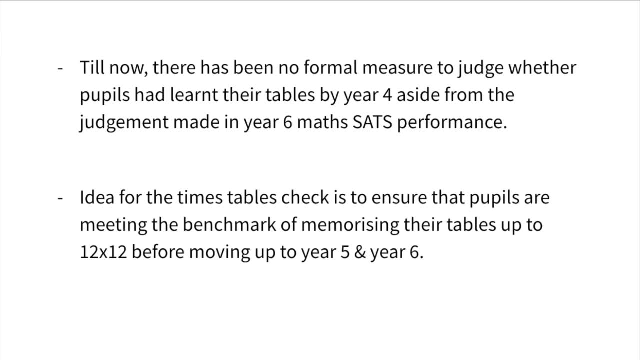 one times tables will be used for practice questions before the test begins. Till now there has been no formal measure to judge whether pupils had learnt their tables by year 4, aside from the judgement made in year 6 Mathsats performance. So the idea for the times tables check is to ensure that pupils are meeting the benchmark. 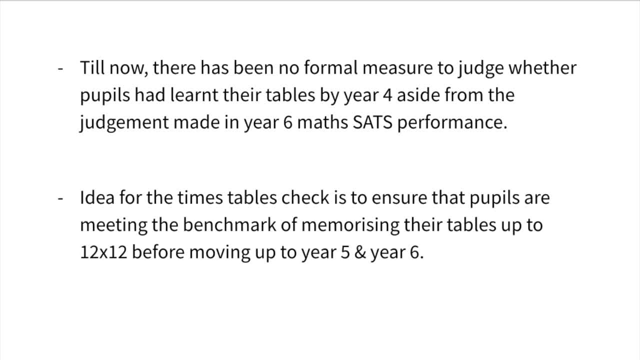 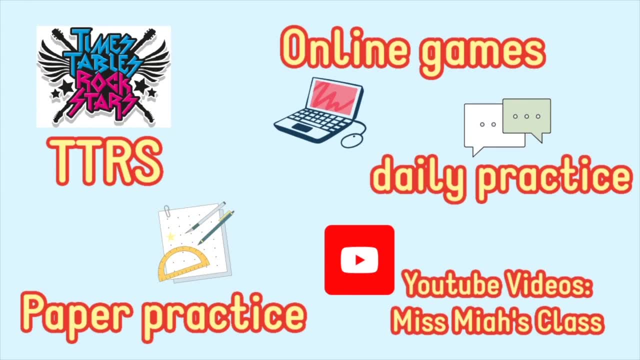 of memorising their tables up to 12 x 12 before moving up to year 5 and year 6.. Here are just some of the ways that we encourage children to practice learning their tables at school. A really good way for your child to practice their tables in a similar format to the test. 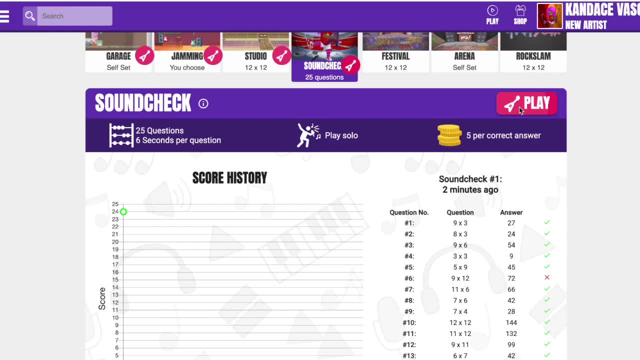 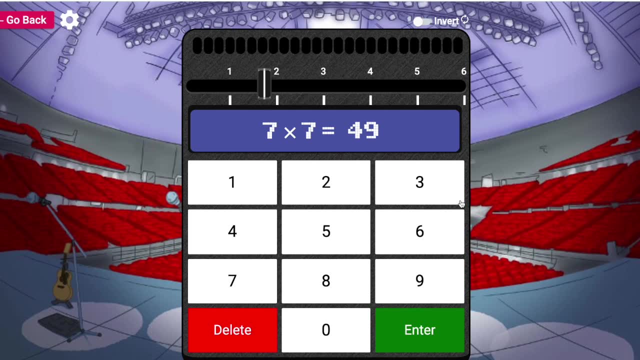 is to log in to TT Rockstars and complete the sound check test. So here is an example of me logging in and having a go at that. So I will be completing 25 questions. This is very similar to what is presented in the multiplication tables check. This is a great way for your child to get practice in typing. 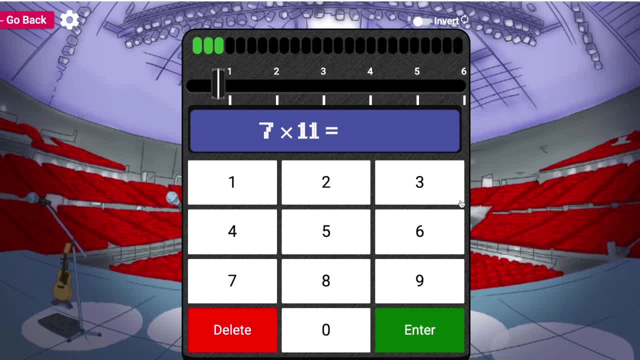 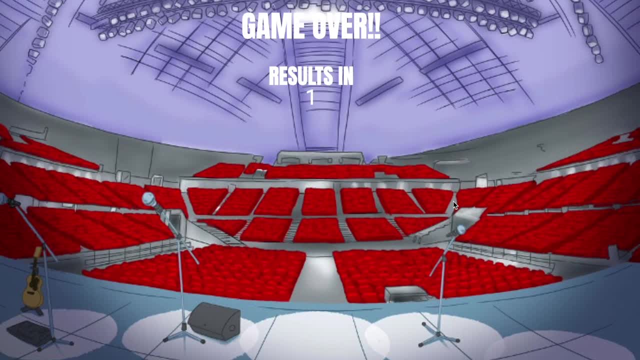 on the keyboard and answering the questions within the given time. So, once finished, your child will be able to start the test. Your child will then be able to see the results and compare themselves to how they did before. A really handy check is the sound check information on the right hand side of the screen. 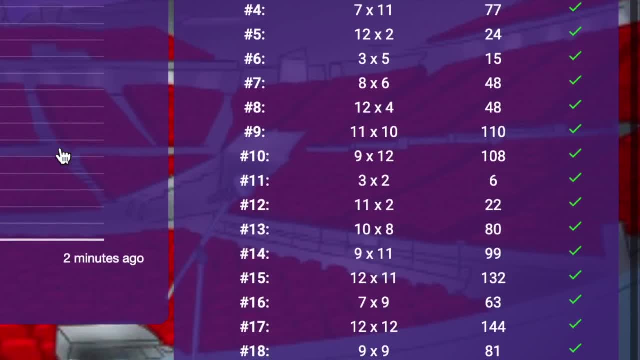 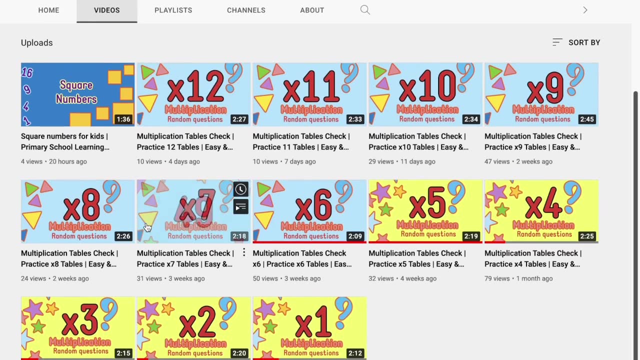 This will help them to see what they have got correct and what they may need more practice on. Another way your child can practice their tables is by clicking onto Miss Mia's YouTube channel. Here you will find short practice videos which are free to use and are great for daily practice. 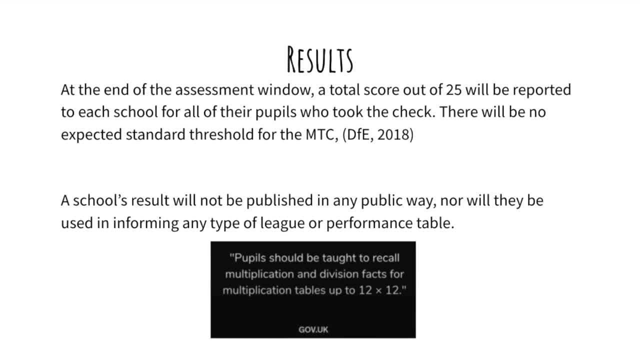 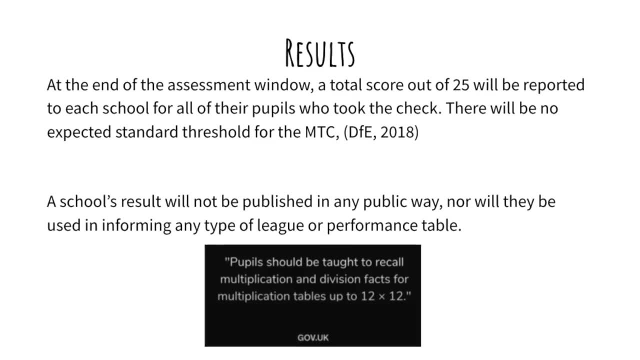 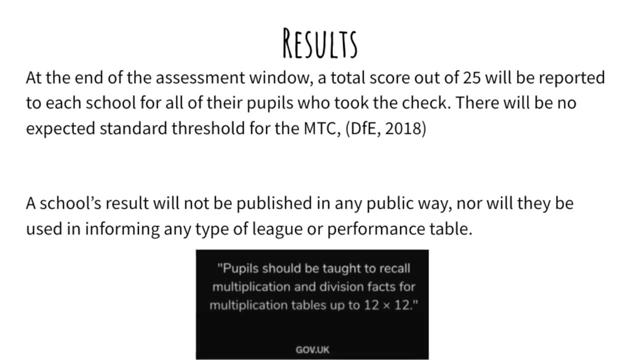 In terms of the results. A total score out of 25 will be reported to each school for all their pupils who took the check. There will be no expected standard threshold for the MTC. The school's result will not be published in any public way, nor will they be used in. 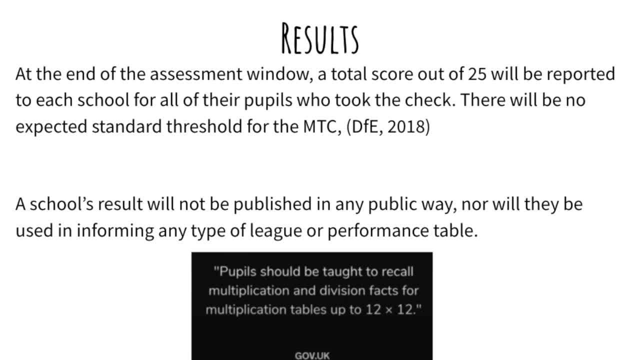 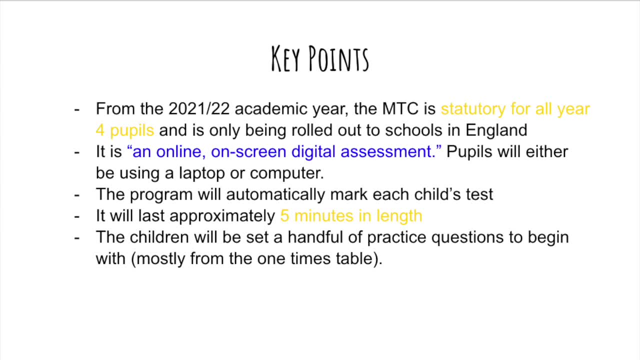 informing any type of league or performance table. So just to summarise, these are the key points From this year. the MTC is statutory for all year 4 pupils and is only being rolled out to schools in England. It is an online, on-screen digital assessment. 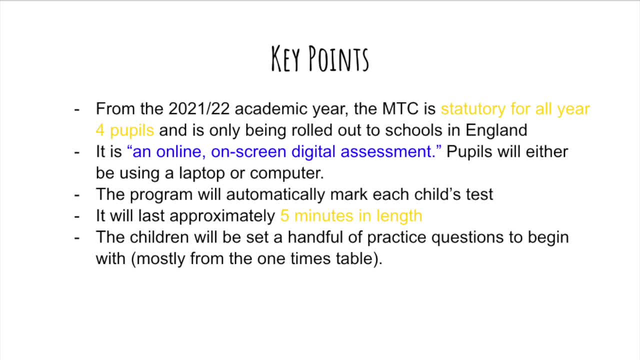 Pupils will either be using a laptop or computer. The programme will automatically mark each child's test. It will last approximately 5 minutes in length. The children will be set a handful of practice questions to begin with, mostly from the one times tables. 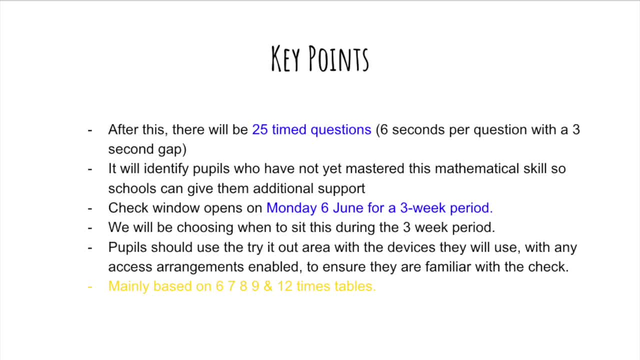 Key points continued. So after this there will be 25 timed questions, 6 seconds per question, with a 3 second gap. It will identify pupils who have not yet mastered this learning process. It will also be able to identify pupils who have not yet mastered this learning process. 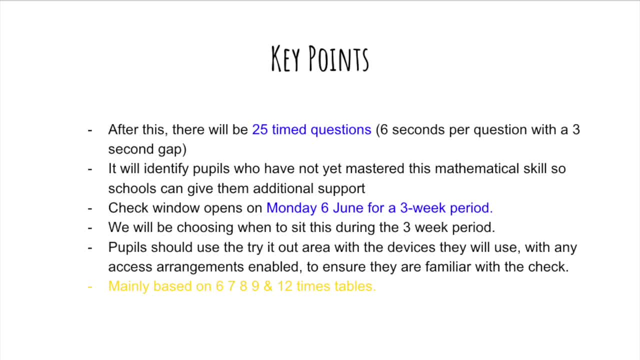 It will also be able to identify pupils who have not yet mastered this mathematical skill, so schools can give them additional support. The check window opens on Monday, 6th June for a 3 week period. We will be choosing when to sit this during the 3 week period. 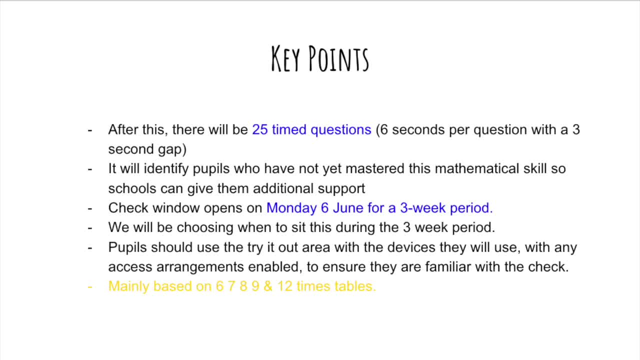 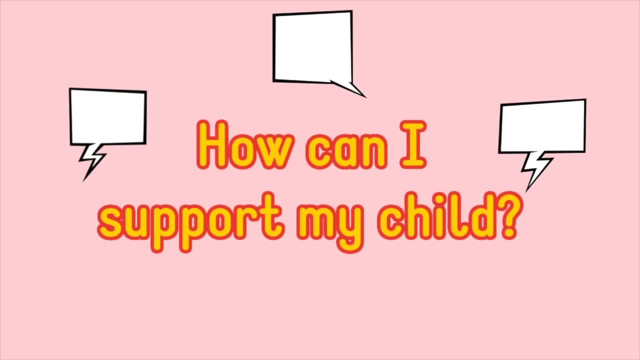 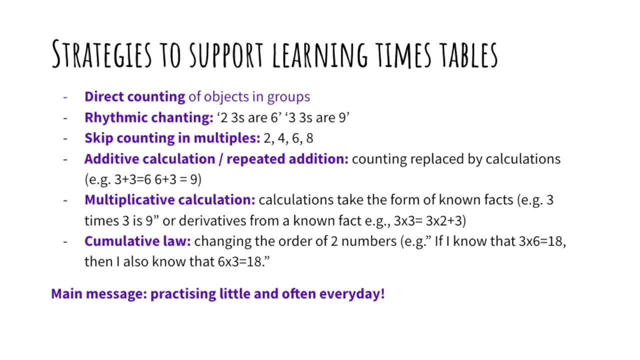 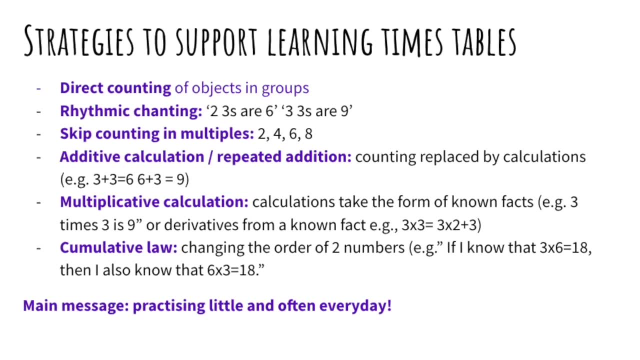 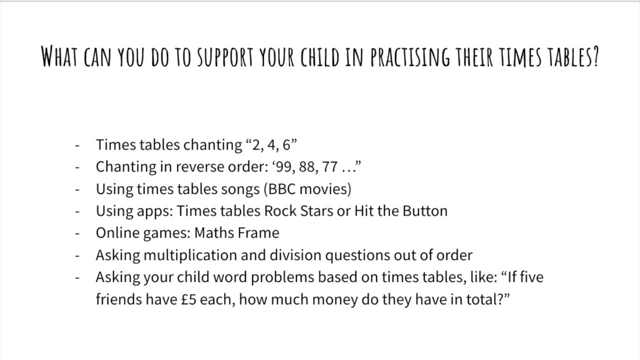 On screen now you will find strategies to support learning times tables with the main message being practising little and often every day. Here are some of the things you can do to support your child in practising their tables. Here are some of the things you can do to support your child in practising their tables.